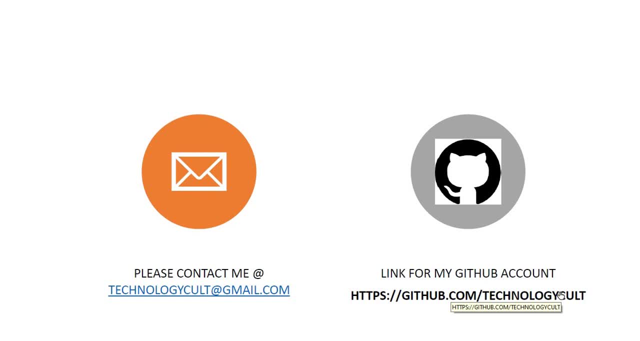 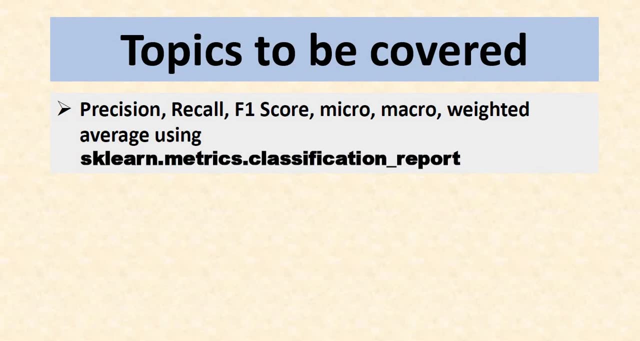 starting. please note you can reach me at technologycurlgmailcom and my github link is also present here. Now topic to be covered is getting a precision recall F1 score- micro, macro and weighted average score using sqlnmetrics. the classification report function: basic. Before that I 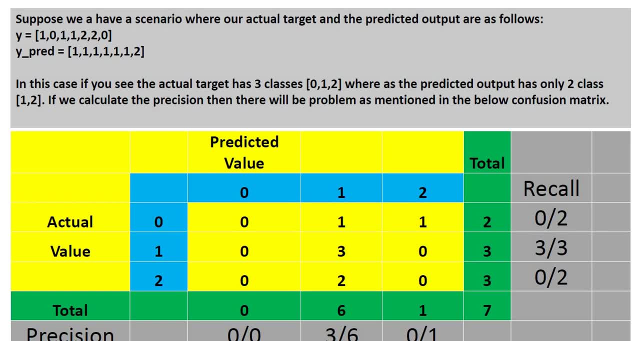 just like give you a like a small description about the error existing error. So suppose we have a scenario where our actual target is: y is equals to 1, 0, 1, 1, 2, 2, 0. we have three instances in our target variable and 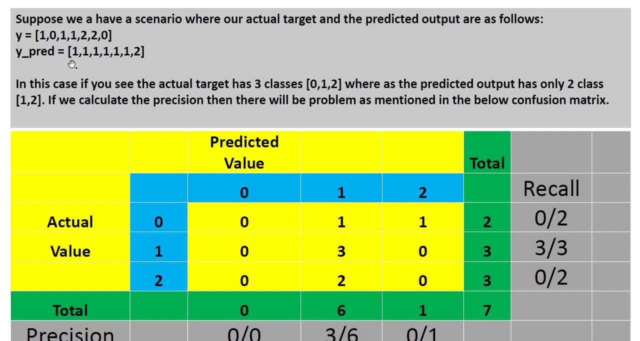 prediction is for two classes, 1 and 2. for class 0 there is no prediction. So, as we can see here, in this case, if you see, the actual target has three classes, whereas the predicted output has only two classes, 1 and 2.. If we calculate a precision, then there will be problem, as mentioned in. 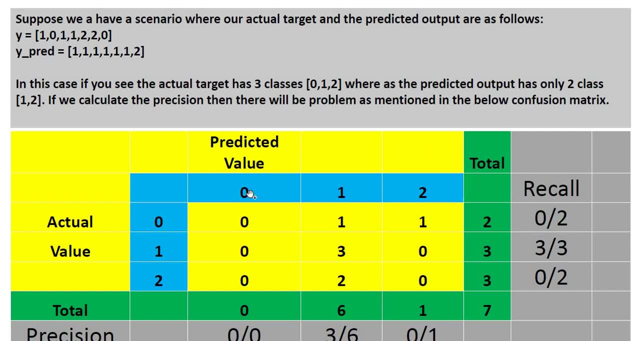 the below confusion matrix: Now, as per this confusion matrix now, if you see here this is my actual value and these are the actual instances of the actual value and these are the instances of predictive value. Now there are 3 class 0, 1, 2 for class 0. the total actual instance will be 2 for class 1. 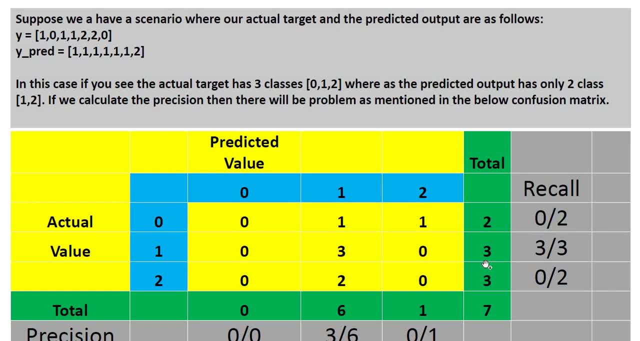 total. some of the total actual instance will be 3 and again 3 for class 2. similarly predicted value, the instance of protected value, is given here and similarly. now, if you want to calculate precision, precision is nothing but a true positive divided by the sum of true positive plus false positive. now for class 0, if you do so, 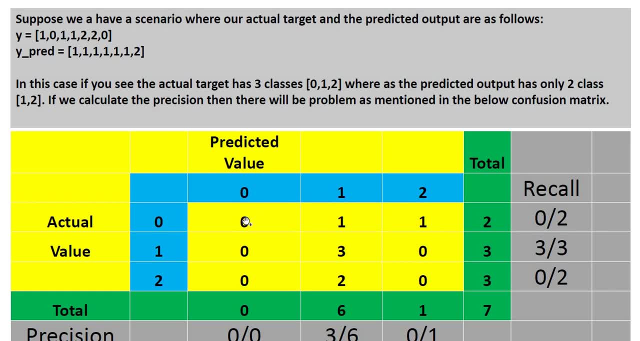 for class if you draw our horizontal and the vertical line. so this 0 here in this cell will be my true positive and this 0, this and this will be my false positive. so precision will be true positive divided by true positive plus false, so 0. 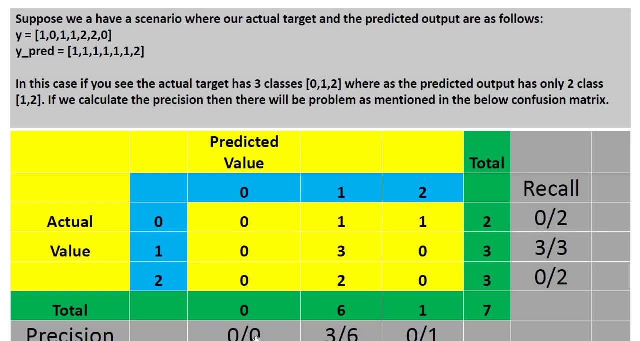 divided by 0 plus 0. okay, in that case it will be 0 by 0 and that will be infinite. we cannot calculate. so when we, if there is such scenario in our program, in a Python, like in our sklearn data set, we have and like we are trying to predict, 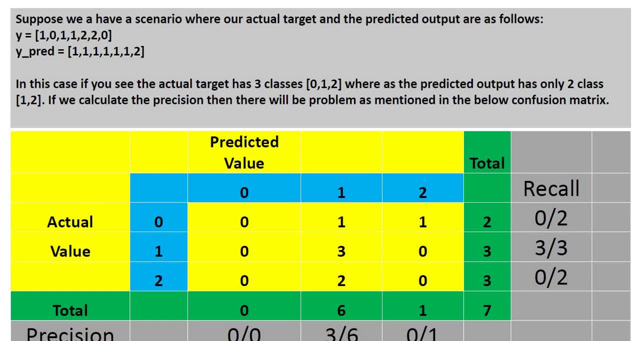 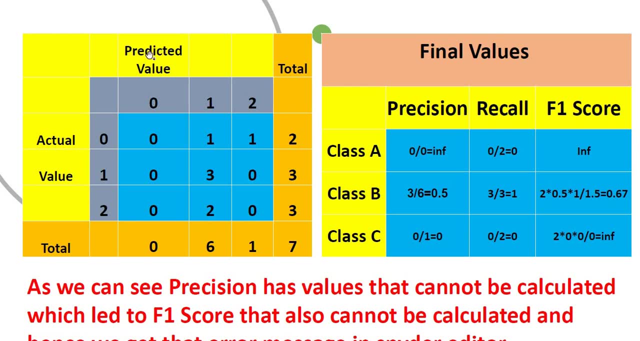 and where we don't get are not a single in predicted value for our class, we will end up getting some kind of error. so I just want to show you that so we can see here the- this is my confusion- matrix and this is the final value. if you calculate here this, 0 by 2, 3 by 3 and 0 by 2 will 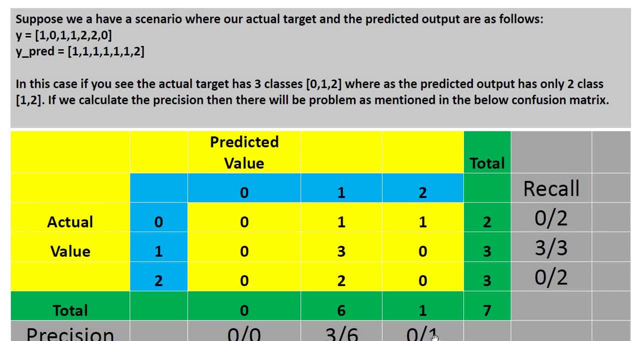 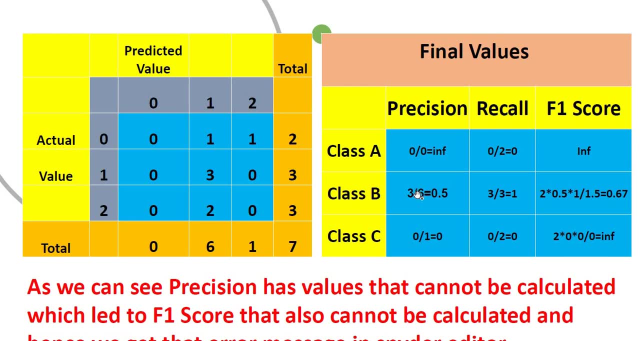 be my recall, and 0 by 0, 3 by 6 and 0 by 1 will be the precision for each class respectively. if you calculate here, precision will be 0 by 0, mix infinity C. for class B precision will be 3 by 6- 0.5, and class C it will be 0 and similarly. 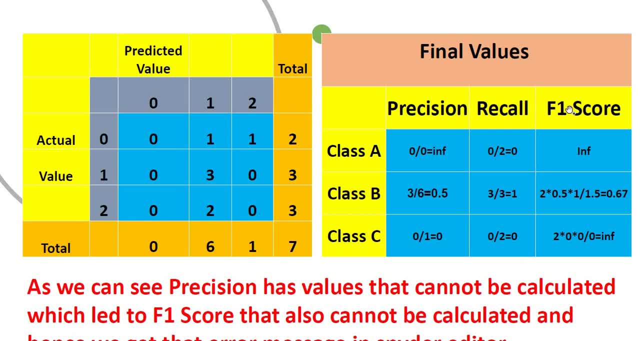 we get a recall now, once we calculate the precision and recall, then only we can get the F1 score, which is nothing but twice into harmonic mean of the precision. and do recall: if a, if the position for class a infinity, definitely f1 score will also be infinity. and then you 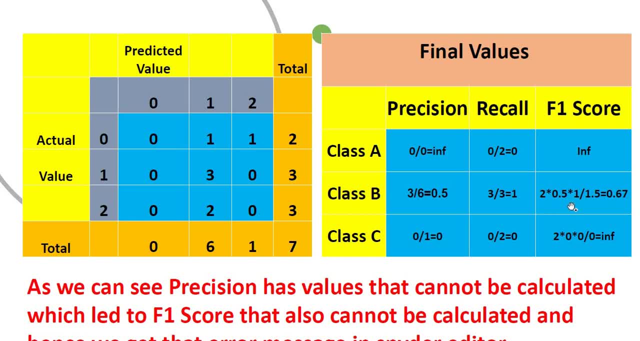 calculate the value for this class b, we get the f1 score at 0.67 and for class c, also will get infinity, because if you calculate this two into precision and to recall, by precision process recall, in this case, for class c, both precision and recall is zero and hence we end up getting 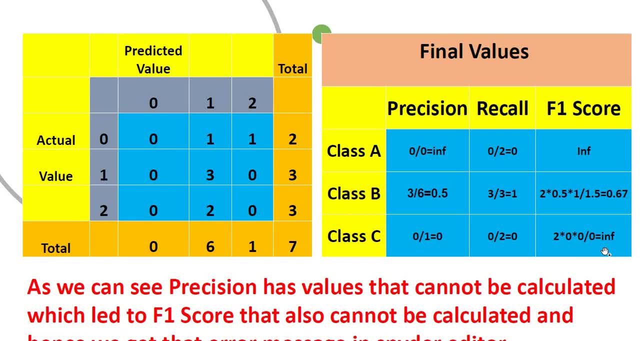 infinity. but how, when we execute this through pi, through a skill and okay, how, what will be the error that we'll get and how we will handle that? okay, so we can see, precision has value that cannot be calculated, which led to f score. that can also. that also cannot be calculated, and hence we get 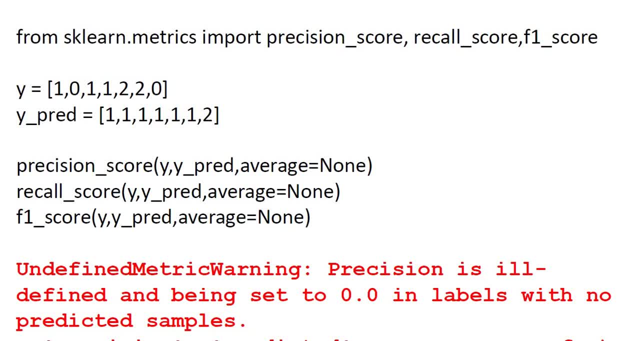 the error message in the spider edition like this: see, i'll execute this person for the time i'm showing you. if you, if you will execute this for precision and for f1 score, we'll get this kind of error. for precision, we'll get undefined metric warning where precision is ill-defined because 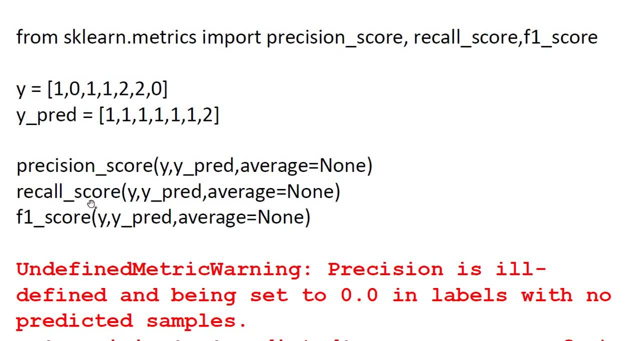 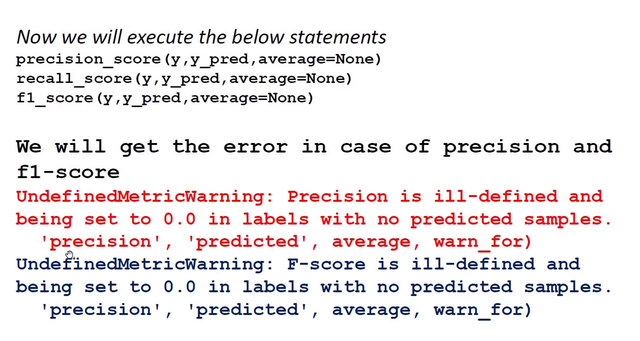 we are getting infinite and when you will execute recall score, it will be executed perfectly again. in case of f1 score, we'll get the message recall f1 score is ill-defined like this, so we'll get the error. error in case of precision and f1 score. precision is ill-defined and being set to 0.0 in labels with 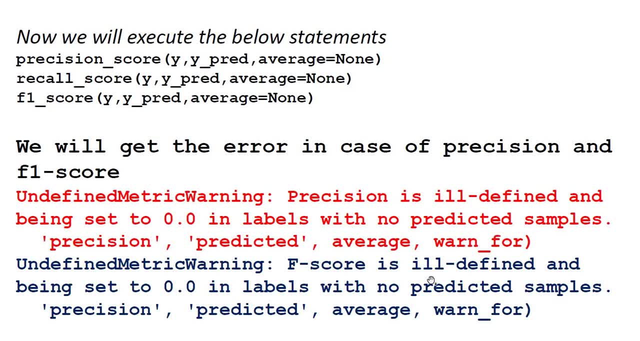 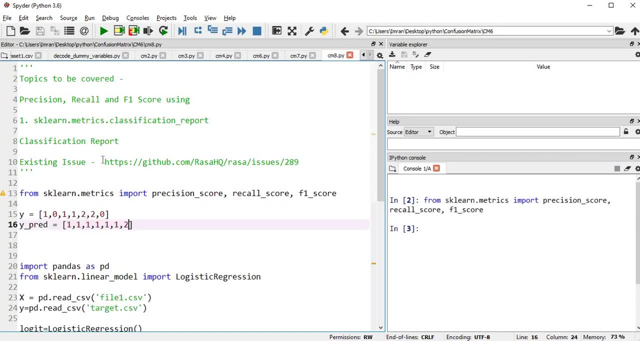 no predicted sample again for f score also, f1 score also. we get the same, the same kind of error, because we are encountering infinite and we cannot calculate that. i will import precision score, recall underscore and f1 score. okay. so if you can see, we don't have. 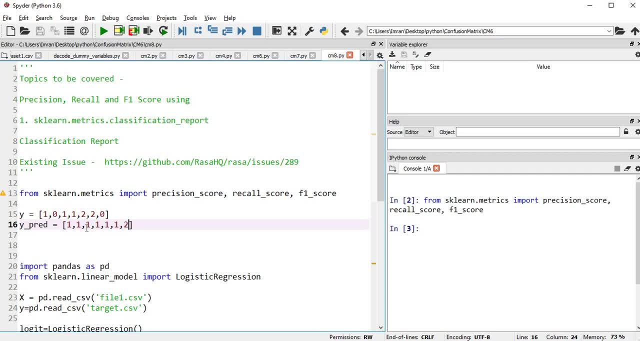 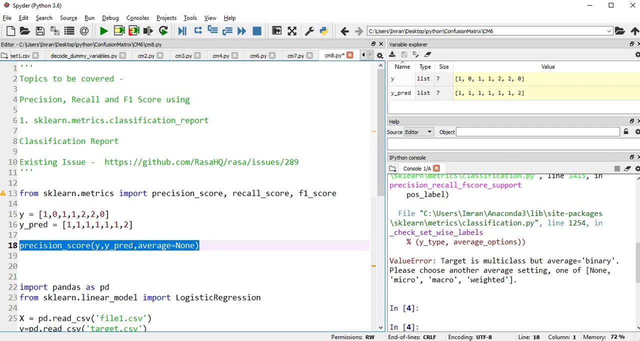 any like in my wipe read: i don't have any instance of the class zero. now what i will do? i will simply, i will try to get the precision. okay, i will pass here so you can see undefined matrix positions is ill-defined because here, if you can, 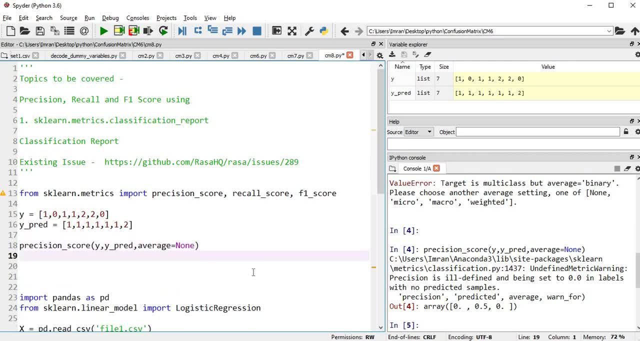 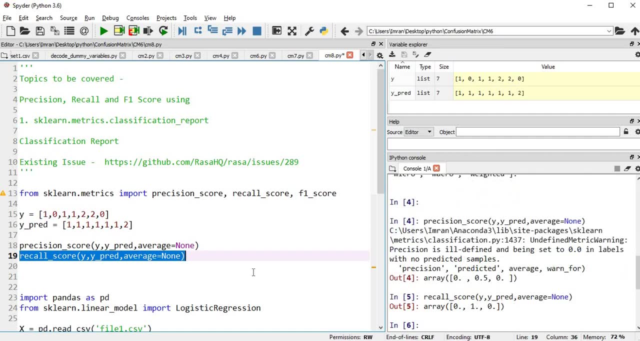 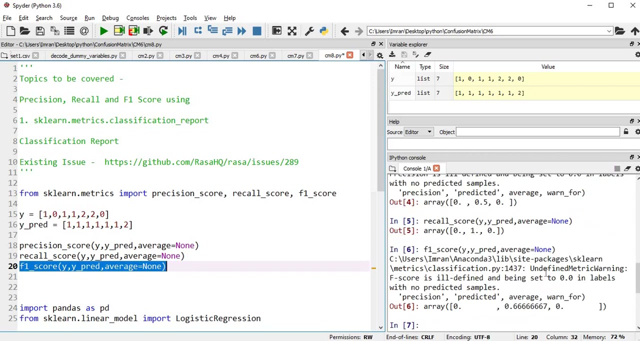 see after that what we'll do. i will calculate f1 score now. you will again see f10 score also. we are getting this undefined metric. f score is ill-defined and being set to zero in labels with no predicted sample. if you encounter any such error, please 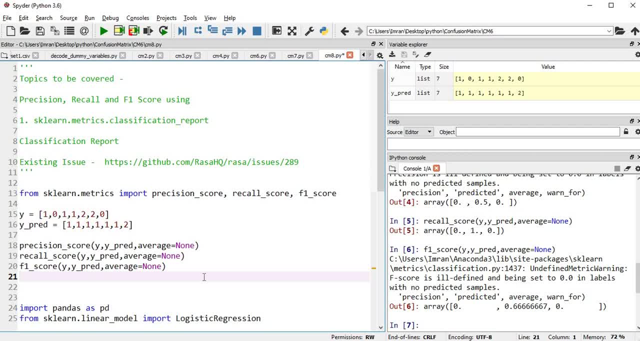 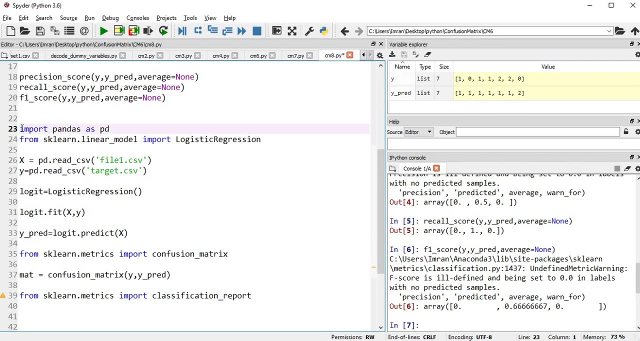 understand that for one of the classes, you don't get any predicted value for one of the classes, okay, or? or the prediction for one of the class is missing, and that's why you are facing this error. let's start with our classification report. so for before starting, classification underscore. 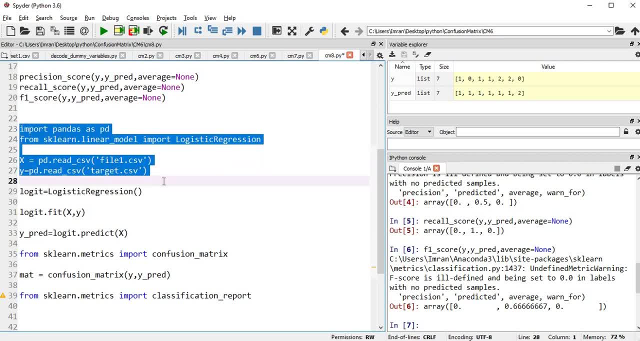 report. what i will do? i will simply: i'll import my data set and then i'll create a logistic regression, followed by fitting the logistic model, uh, logit, and then i'll predict it and then i'll create a confusion matrix and then i will import- uh- import a classification report. so my confusion. 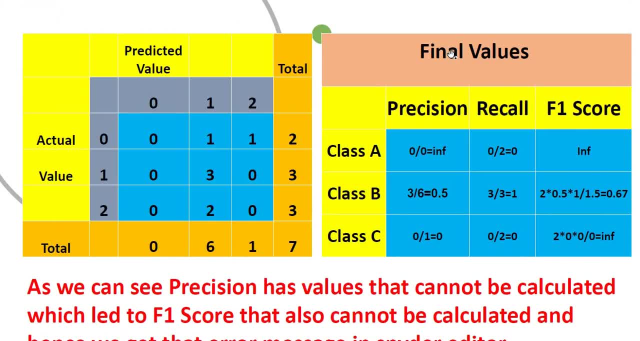 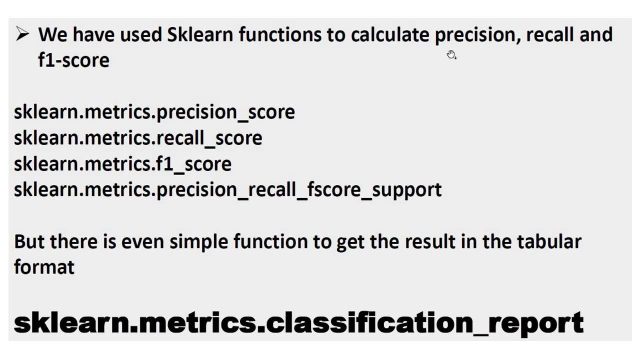 matrix created. so our main target is: whatever we have created. okay, this is see. why i want to show this is because, see, we have used a scale and function to calculate the precision, recall and absence. so we have used a scale and dot matrix or precision underscore, recall underscore: f1 score. 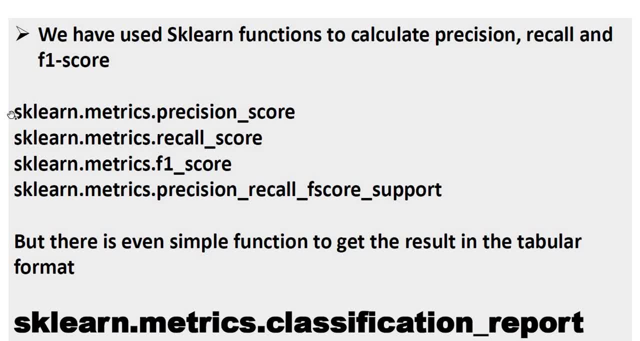 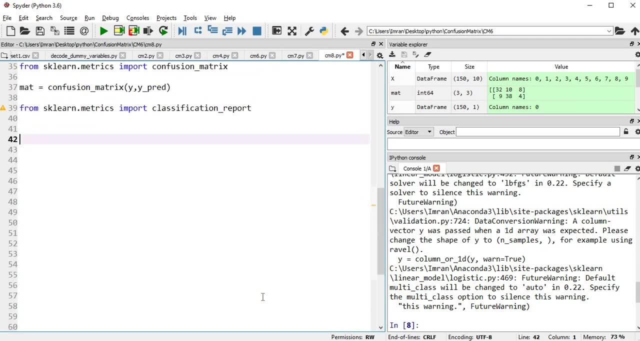 even precision, underscore, recall underscore, f score and support, but we are not getting the proper tabular format, the one step shop, i mean to say. so that's why i will use a skill on dot matrix, dot classification, underscore report to achieve the same. i will simply, i will simply print a classification report. 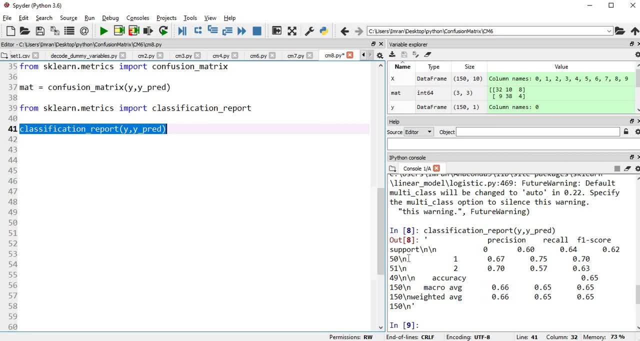 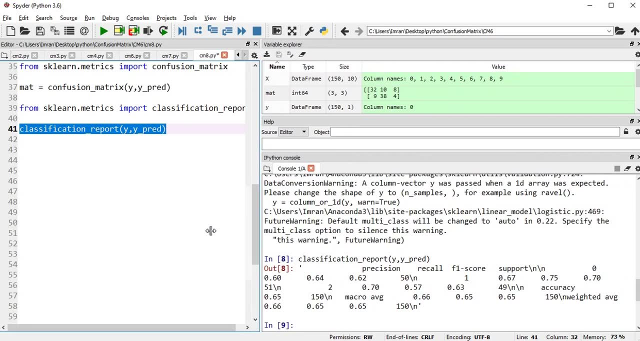 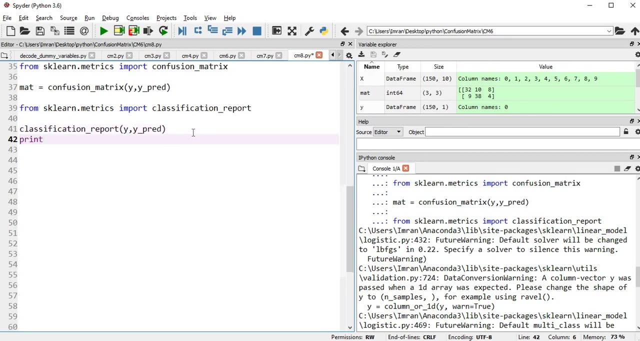 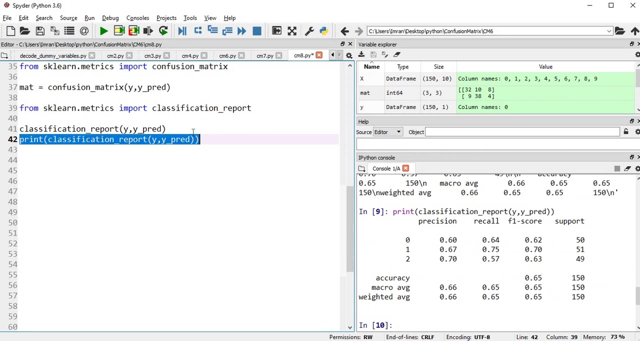 so if i do this, okay, so you see, this value is not that readable. okay, it's very difficult to read this like it is coming but not properly see here. so what i will do instead of this: i'll copy this and then i'll print. now you see, it is coming proper, right, but again, if you see, uh, what i have said, that 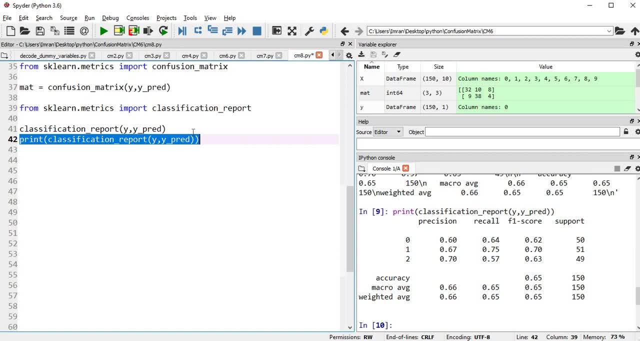 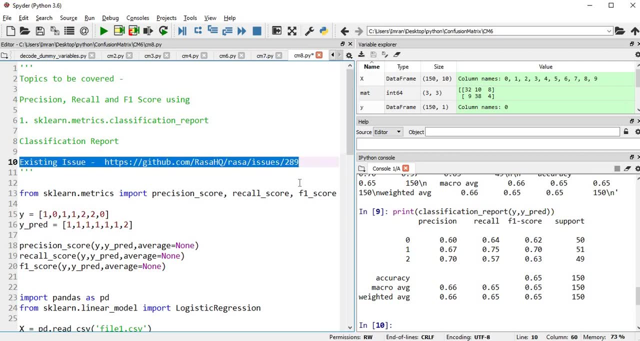 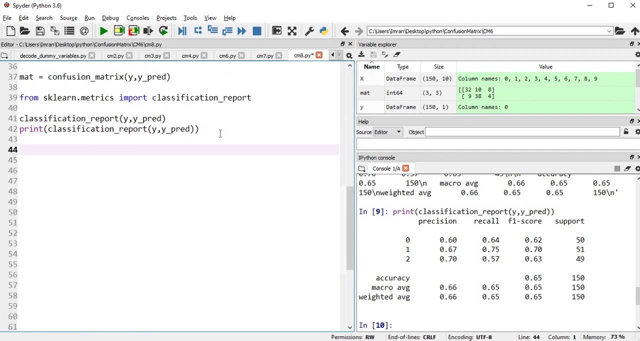 we will print the micro average magnet, but micro average is missing. there is an existing issue with this classification report. you can- i will mention this in my uh description, uh of my youtube, wherein you can get this and you can view what is the issue. but i'll show you what is the issue, okay. 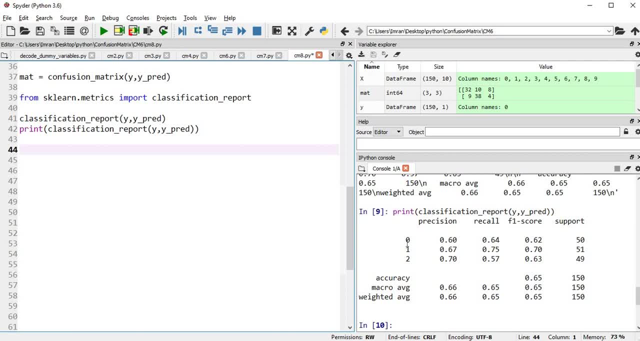 so what i will do now? uh, if you see here zero, one, two, i do. i'm not contented with this zero and i want the class a, class b and class c. so how will i achieve that? okay, now what i will do. i'll get this. 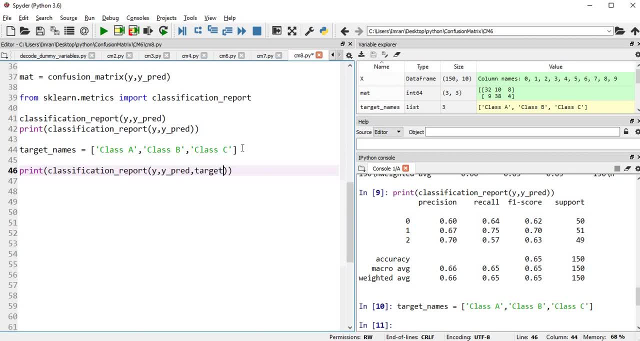 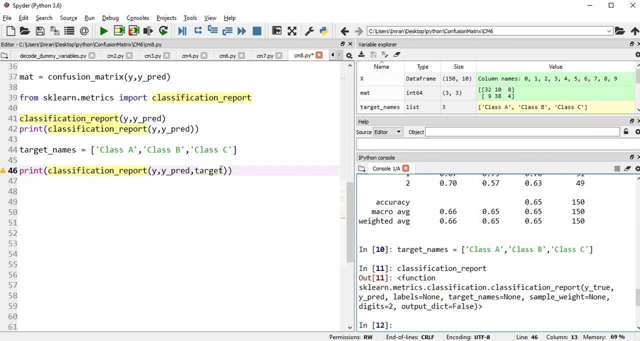 and then i'll pass this, the parameter target. you give here control, i, okay, or you just you print here classification, okay. so these are the parameters that can be passed to classification report. so in this target name it is none by default, so i'll pass target name. 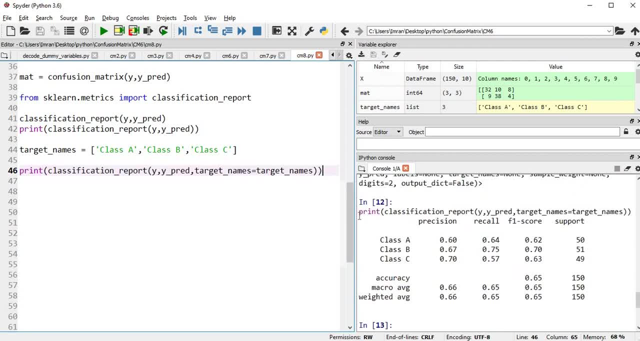 now this zero one, two is being replaced by a, b and c, but still we don't. uh, i don't see the micro average. okay, if i want to see the micro average, what i will do, i will, i'll pass the label there. one comma two, comma three. okay, if you see, here my labels are. 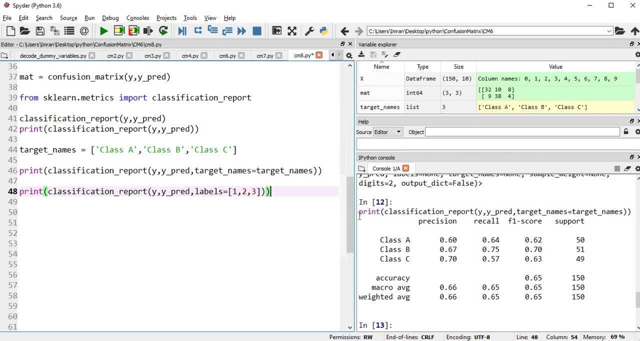 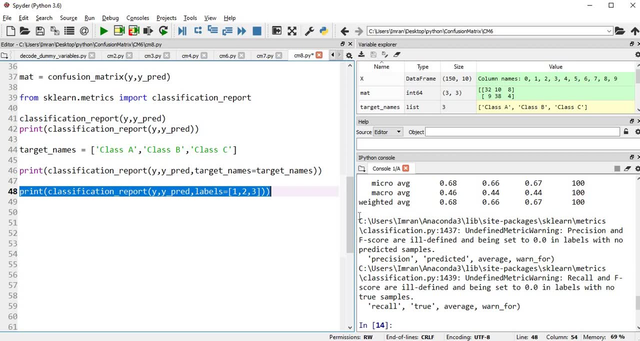 actually zero, one, two and what i'm passing? the labels one, two, three. if i do that, i'll end up getting this error, because this is the error which i, which i have generated myself to show you how a skill and will behave. if you see, here we get the micro average, we get the macro average and 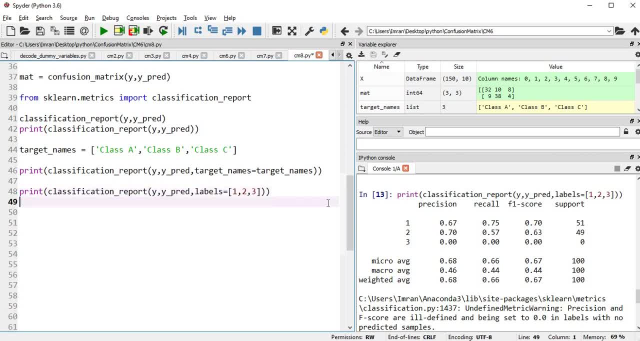 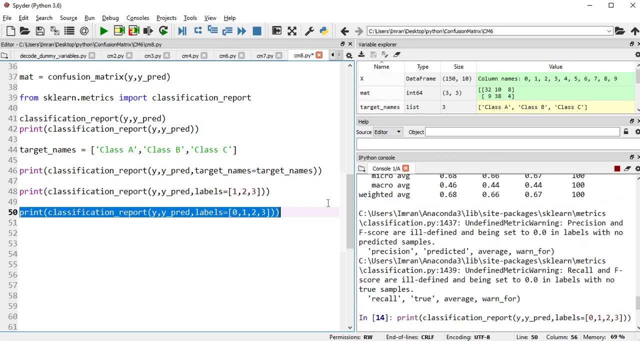 the weighted average, but we don't have the class zero in order to achieve that. what you do? you trick sklearn and you pass zero also okay, and now you execute this. so now it is executed properly. only this three is coming, which you can ignore, and the rest. 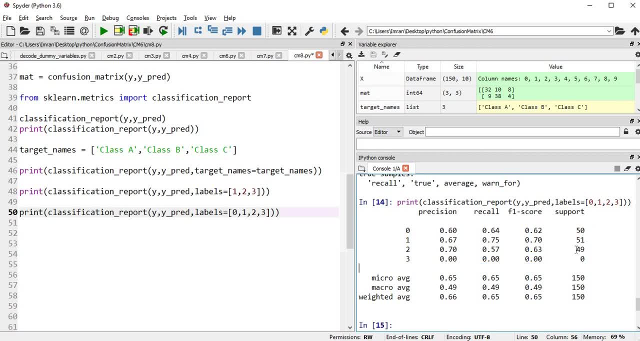 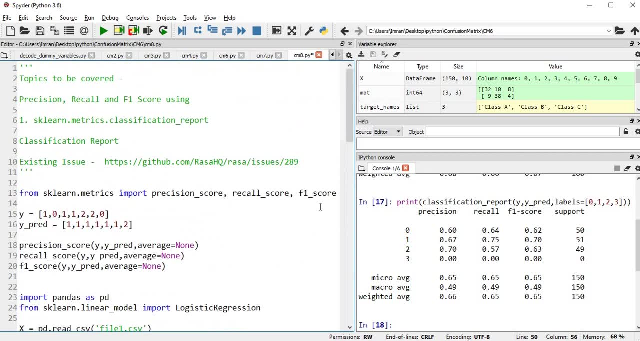 everything, whatever value, precision, recall, FN score and support. everything is coming as per our report, which we have calculated previously. so if you see so, thanks a lot for watching the session. I hope you have understood the error we get when we don't predict one of the classes. this basically happens when we 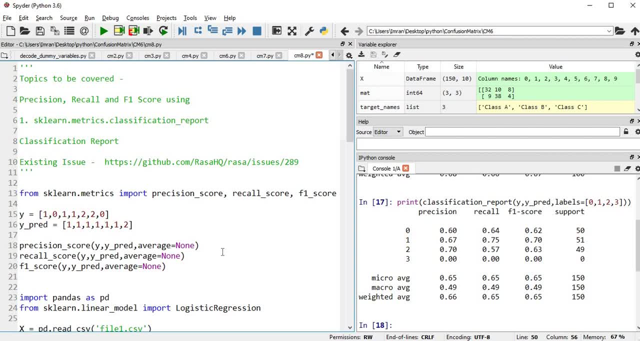 have the imbalance class. okay, in those cases, suppose we have a class in which there are we have 100 records in which for class, in our output variable there will be two classes. so in balance class means we have for one instance of the class we have 90 rows and for the other instance we have 10 rows. so these are. 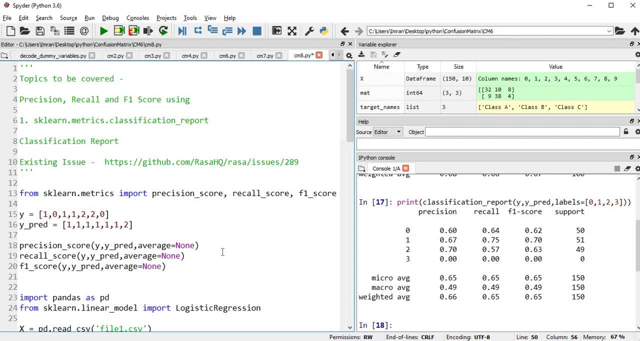 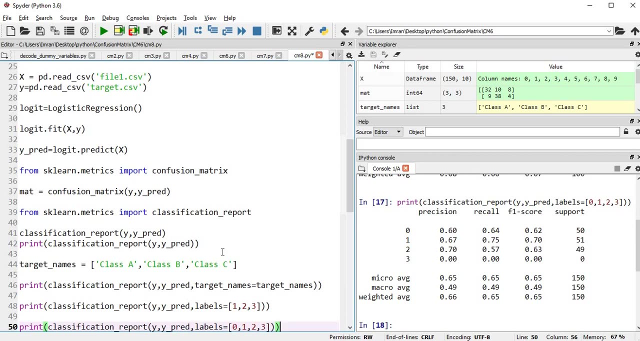 the typical examples of imbalance class. so in this session I have shown you the error, that is, error which is related to error which is related to the precision score- a, a, a, a, the precision recall and FN score. again after that I created a logistic model and then I what I've done, I've imported the classification report and then I have 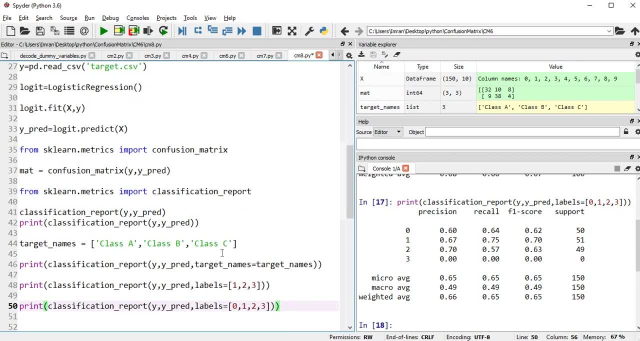 like, shown you how to avoid the error by adding one class, though it will not impact the score for precision, recall and FN score, and we can execute it properly. so thanks a lot for watching the session. if you feel this video is helpful, please press the like button and subscribe to this channel and I will see. you in the next video. thank you. 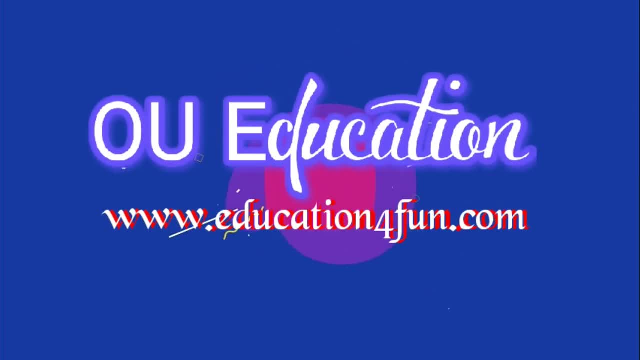 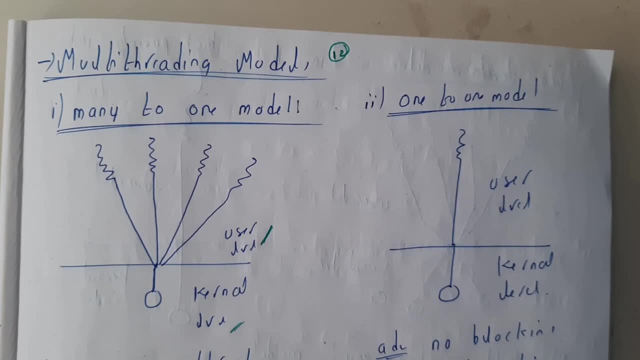 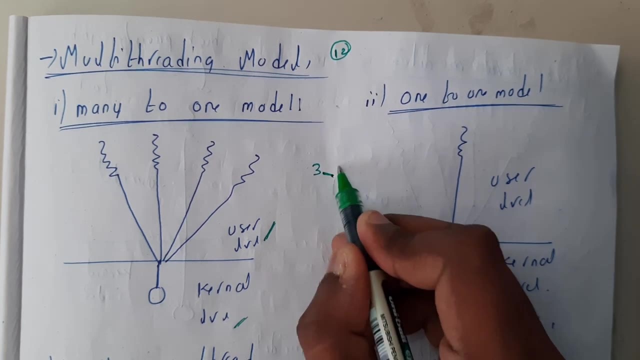 Hello guys, we are back with our next tutorial. In this tutorial, we will be going through the multi-threading models. So, basically, these models are divided into three types, whereas the third type is further divided into one more type. So basically, this is. 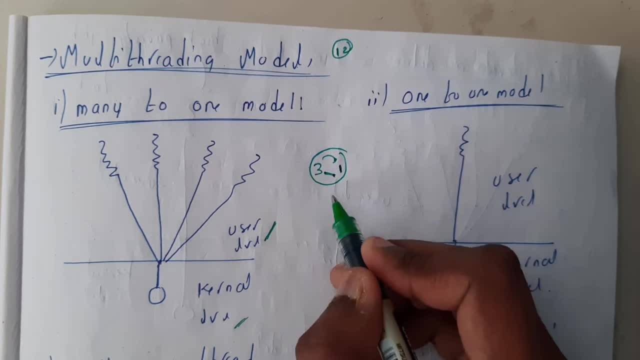 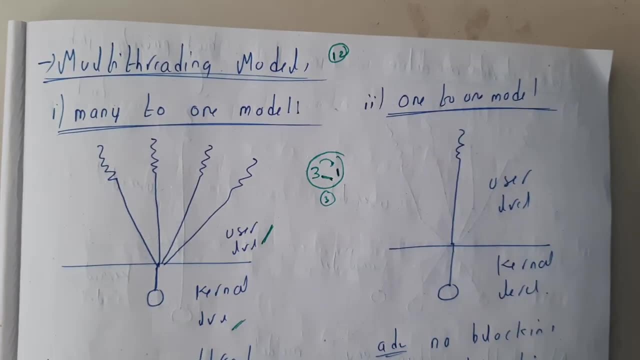 an updated version of third type. So basically, in total we are having four. but in any competitive exams or anywhere, please mark the option three itself. Fine, Okay, So many to one model. So many to one model is nothing, but when a user is creating n number of threads and